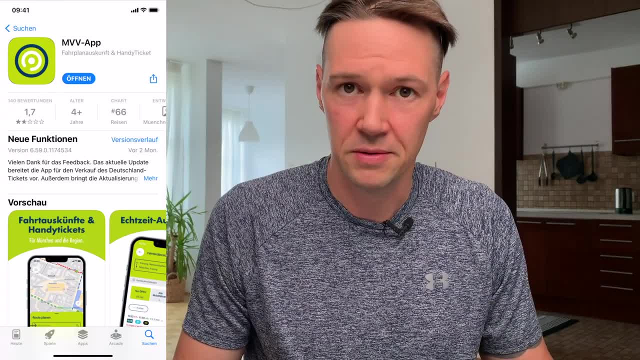 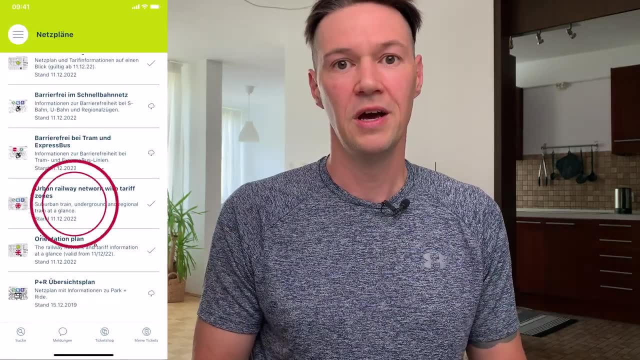 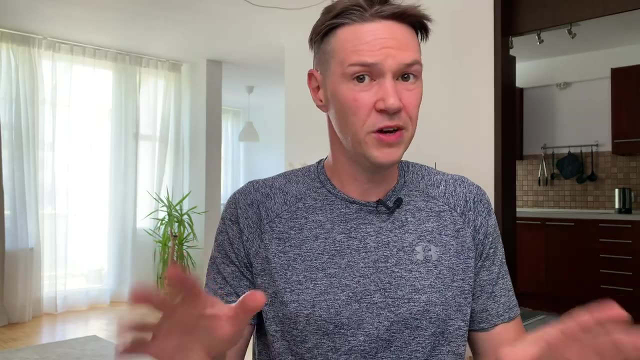 Okay, It's like Google Maps, but better. But what is more important, this application has all up-to-date routes of all public transportation in Munich and you can save them in PDF format or use them directly from this application. This is very useful stuff. Now about transport itself. 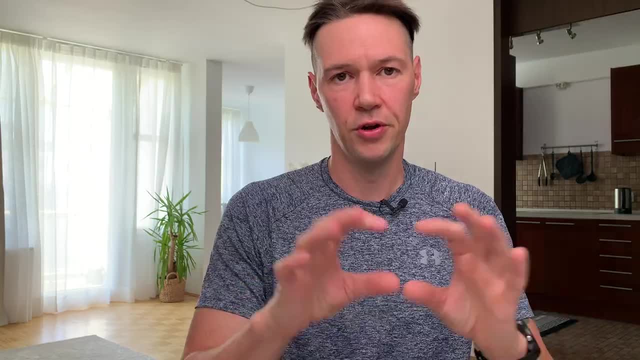 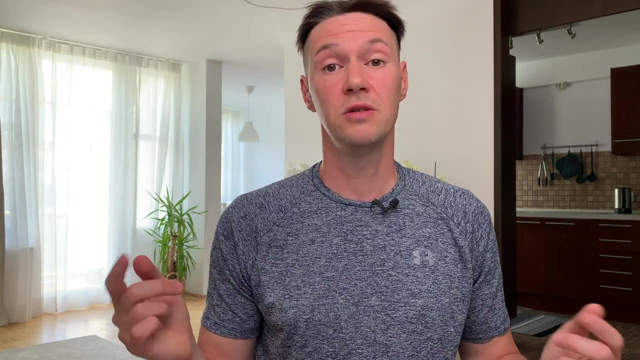 All public transport in Munich has following information on its number of the route and ending station. Number of the route is clear, but ending station probably requires some additional clarification. First of all, it tells you the direction where this transport actually going. This means you. 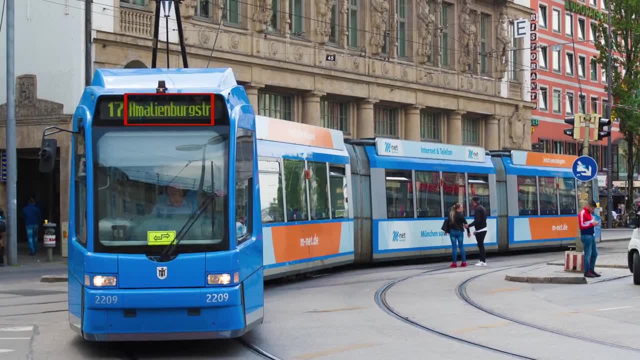 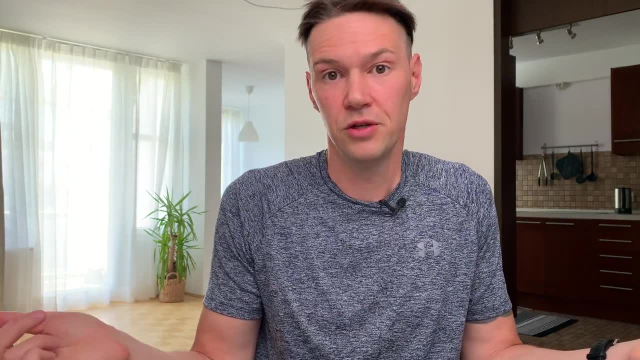 need to know ending station of the route you are going to take. And guess what? Yes, Here you need this application with all route plans And there you will see all the stations that you need. At least I did so five years ago and nobody laughed at me. 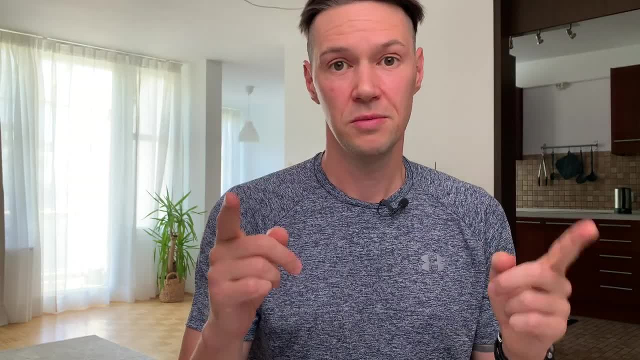 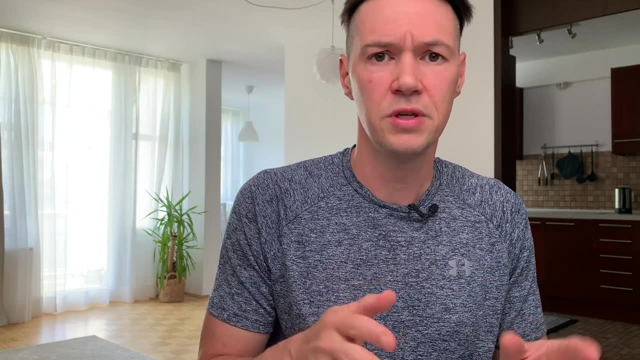 Another important thing: Ending stations may change Because of, let's say, route optimizations in Germany. because of, let's say, route optimizations in Germany. because of, let's say, route optimizations in Germany, many of the routes have short and long versions. Another situation is some buildings happening. 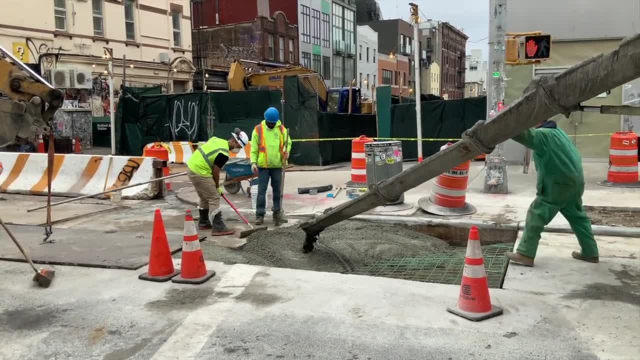 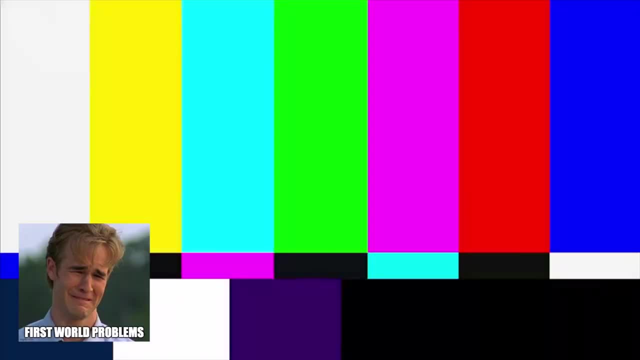 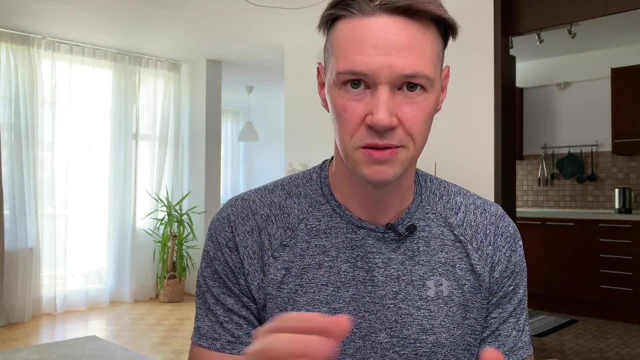 and this transport simply cannot go through some specific place. How are you going to get to your location? in this case? What can I say? Life is pain And it's Germany. You have to suffer, But you can get a bit of pain relief with these small hints. 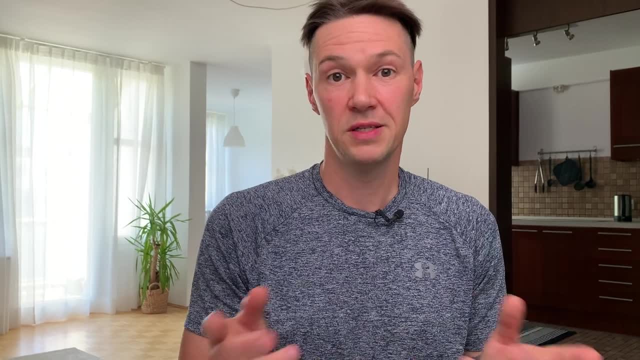 First of all, when some of the important routes is broken, and this happened, by the way, pretty much often. First of all, when some of the important routes is broken- and this happened, by the way, pretty much often. First of all, when some of the important routes is broken, and this happened, by the way, pretty much often. 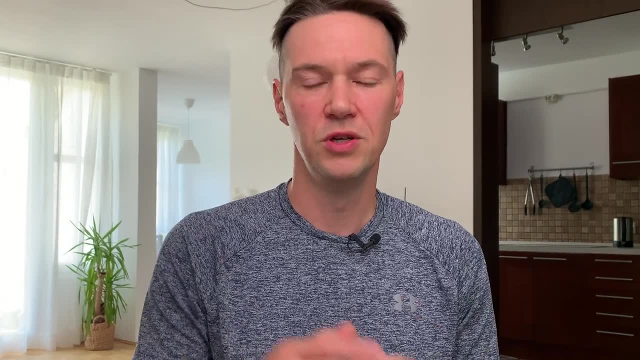 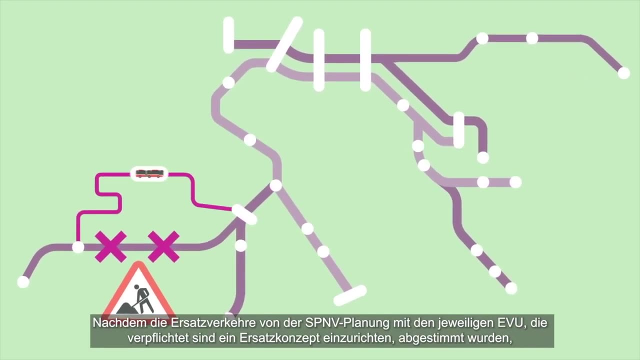 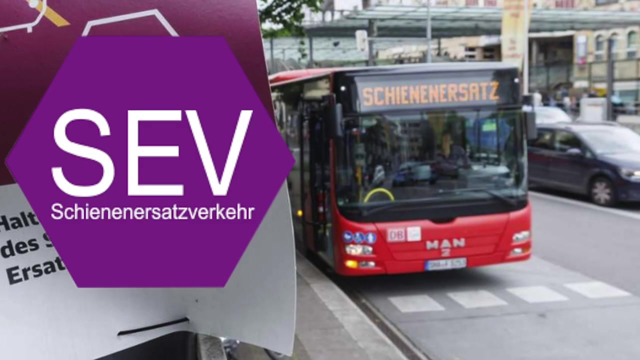 the city provides you with some additional transport which connects the broken parts. For example, it can be a bus which picks up passengers from last available station and simply brings them to next available station. Usually, such buses are free. This transport has sign SEV, which stands for Scheinen Ersatz Verkehr. 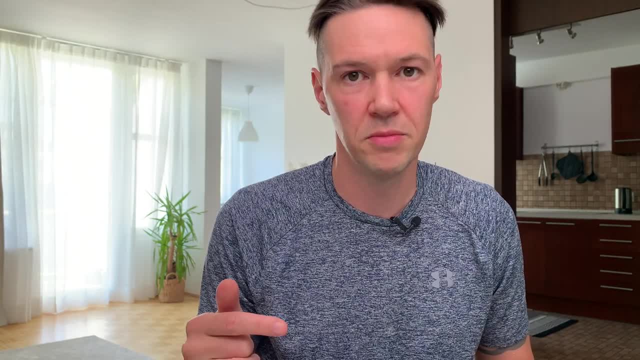 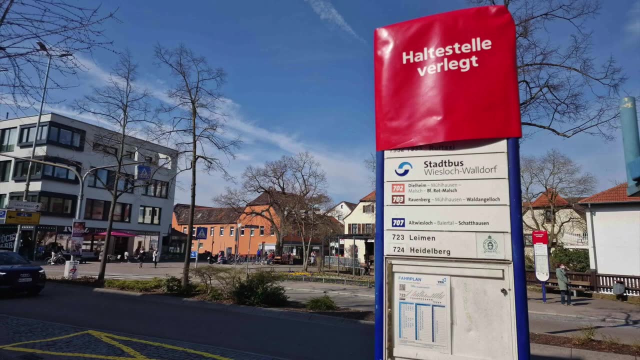 Probably this time I read it correctly: Probably yes. Another thing: you need to know that sometimes when you come to some station, you can see an orange case on the sign of the station. This means you are lucky today and the station is not being. 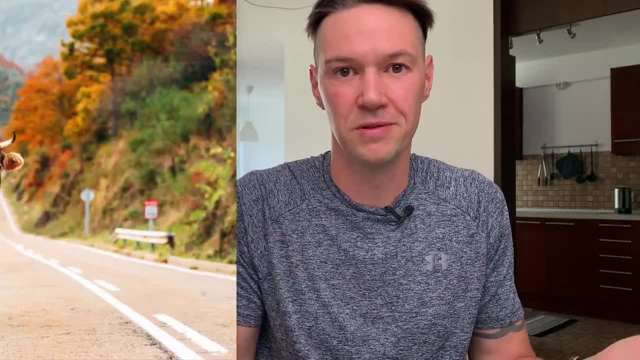 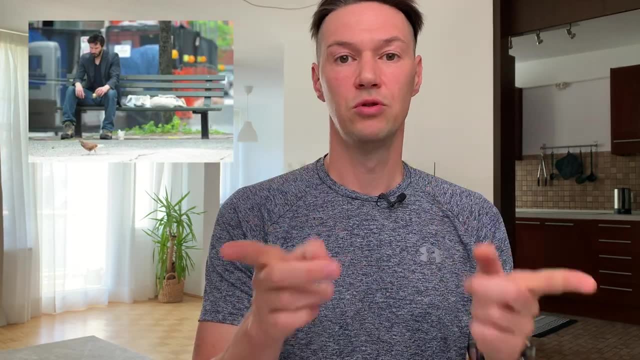 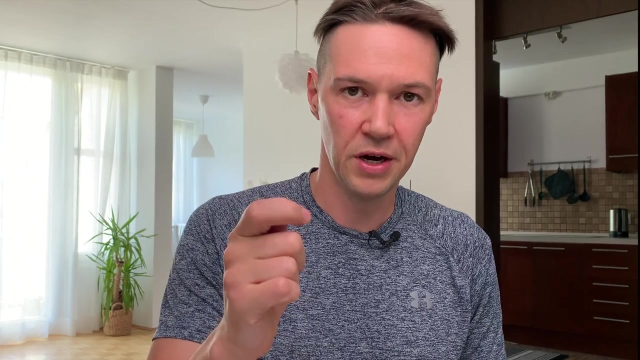 served by public transport because of some- I don't know- problems. What you can do, first of all, you don't need to wait, Nothing will come, But what you can do is read instructions on the station itself. It's usually written in German, so you will require your patience and your mobile phone with. Google Translate. But enough about bad things. There are also very good things, And one of them is that German public transport- I mean S-bands and U-bands- they are working at night. Yes, the whole night. They have bigger intervals, approximately 30 minutes. 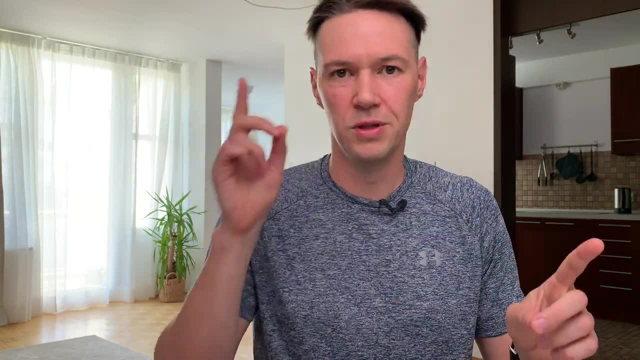 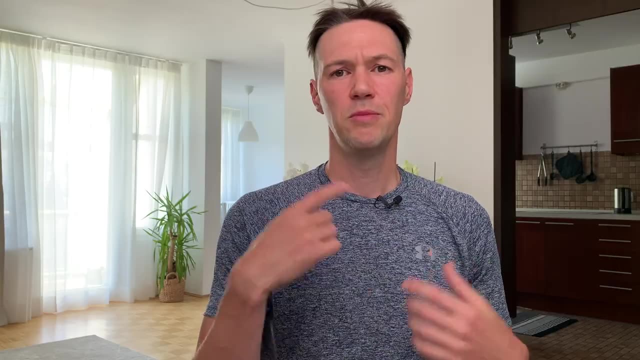 But you can be sure that you can go from point A to point B at night also, And you don't need to take a taxi for 50 euros. Now I'm going to tell you more about Which transport is available in Munich. So first one is U-Bahn. 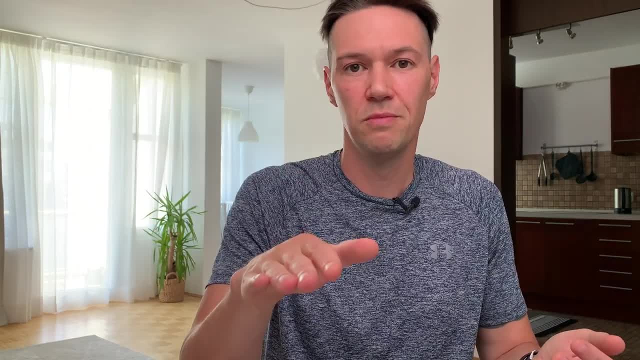 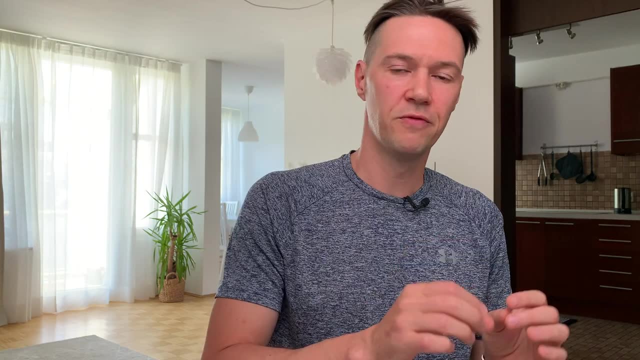 It's like metro, I don't know. It goes on the surface mostly and covers only city area. I can say that this is pretty much reliable way of getting from point A to point B. It goes very frequent and usually does not have a lot of interruptions. 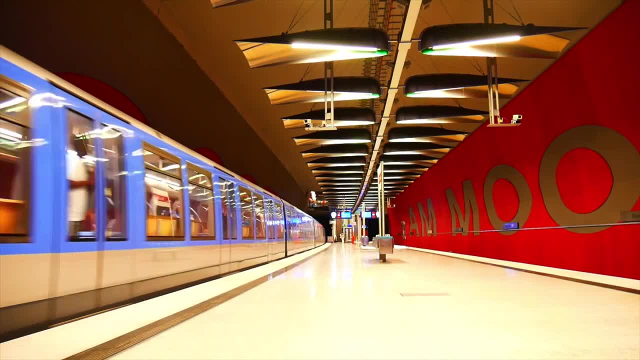 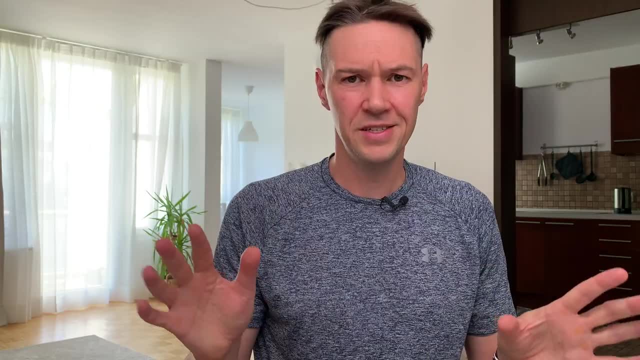 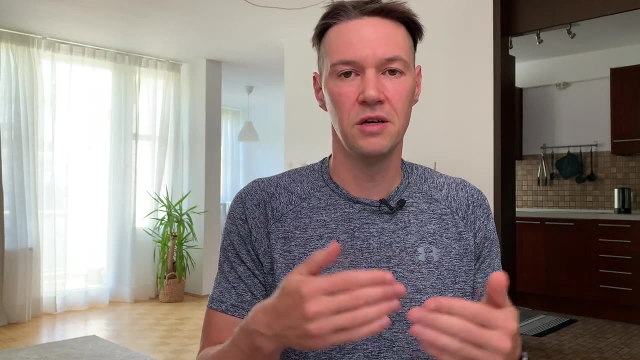 In busy hours it has pretty much frequent intervals, Something like five minutes, And for example, during nights it's 30.. Another thing is S-Bahn. S-Bahn is actually suburban trains which are integrated into U-Bahns, So there are some stations which can use both U-Bahns and S-Bahns. 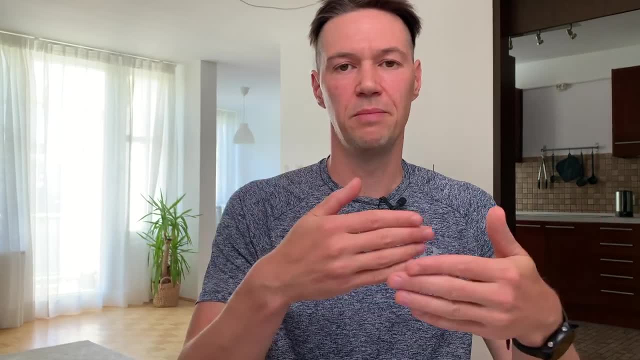 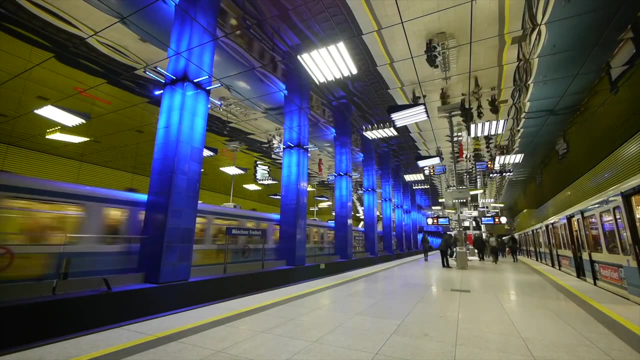 But S-Bahn and U-Bahn never arrive to the same platform, Meaning that there are separate platforms for S-Bahns and separate platforms for U-Bahns. So if you need to change one of the transports, you need to go to other platform within this. 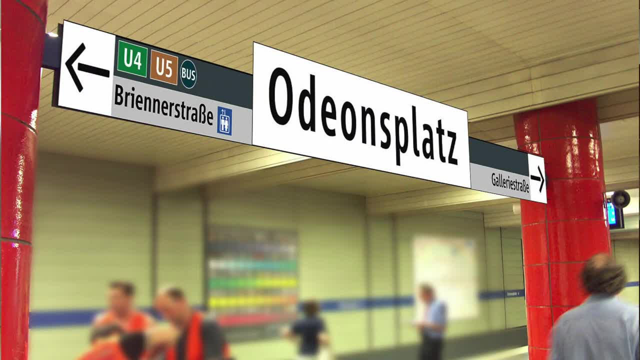 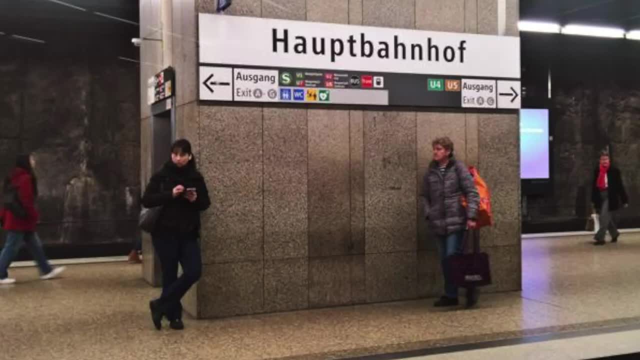 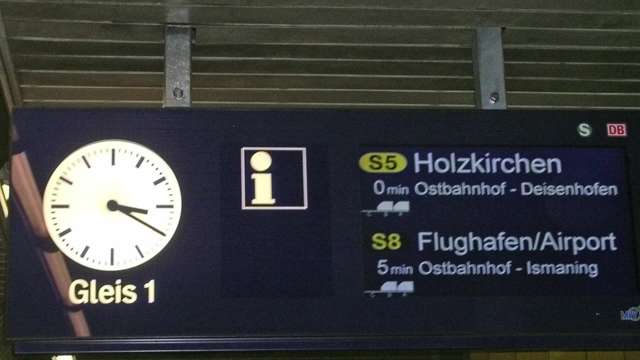 station. So follow the signs, usually on the walls where to go. Usually they are pretty much clear to understand. There are simply like arrows with the numbers of, like S and some number This is S-Bahn route and U and number It's a U-Bahn route. 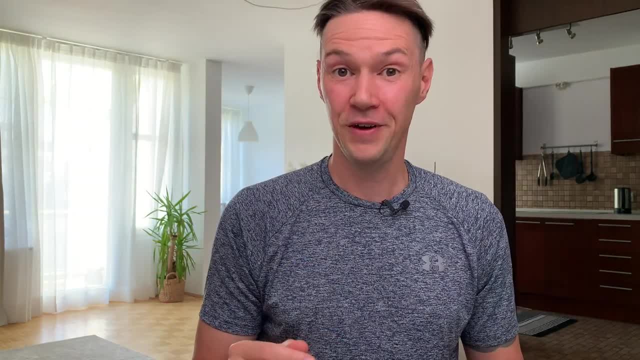 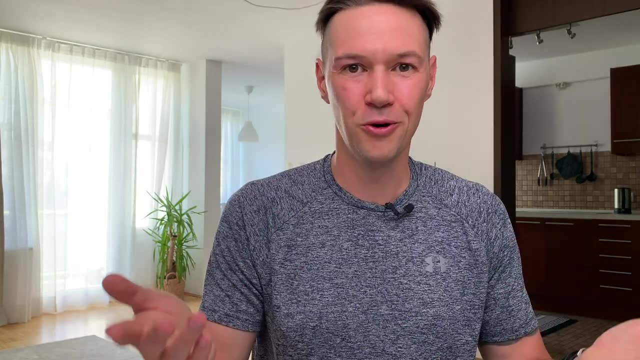 Follow those signs and you will find necessary platform. Fun fact: The first city integration exam for newcomers is to change S-Bahn to U-Bahn on Hau-Bahnhof Station. Good luck. I even heard about people who were lost forever. 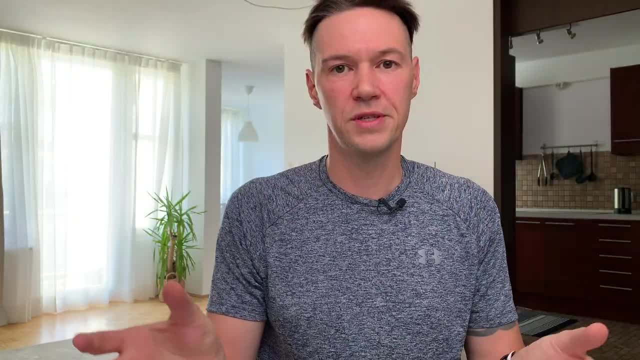 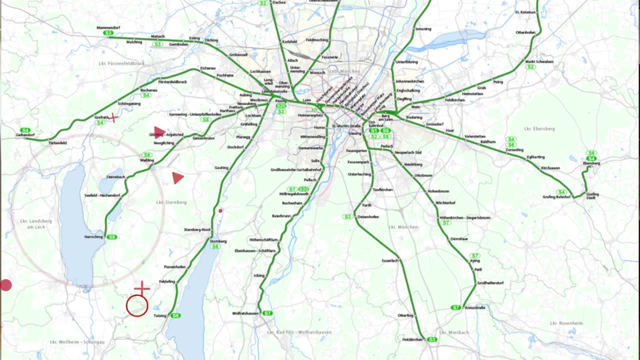 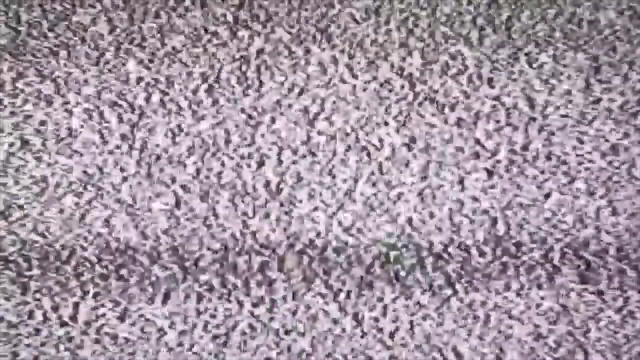 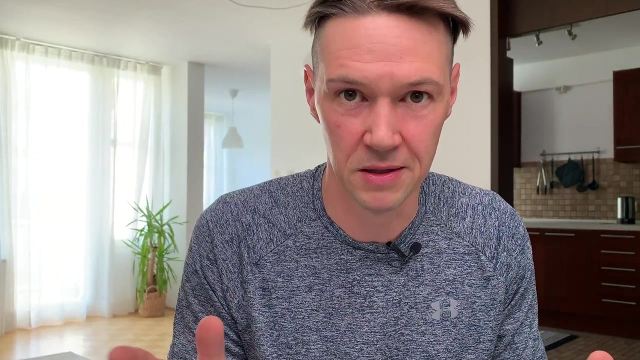 What is cool about S-Bahn is that they cover also suburbs of Munich, And it means you can go with S-Bahn to pretty distant location and to a lot of recreational zones Or, for example, to Munich airport. German famous precision somehow disappears when it goes about S-Bahn. 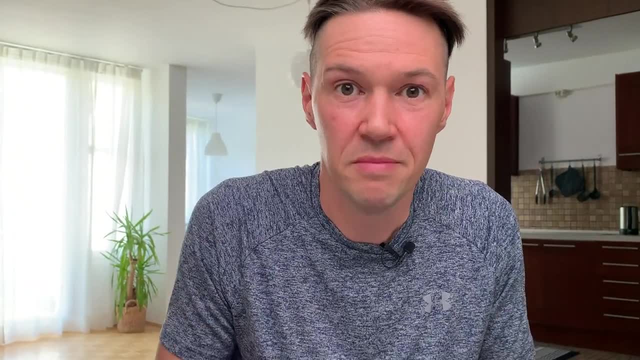 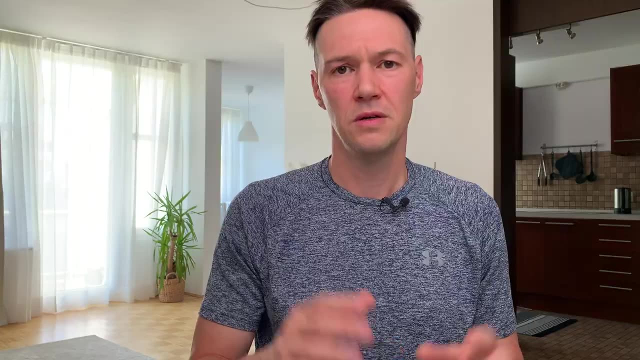 I don't know. Maybe it's some kind of disease, Maybe there are some pills against it or some medical treatment. I don't know. This is unclear. So again about S-Bahn: if you are not looking for new adventures, be careful. 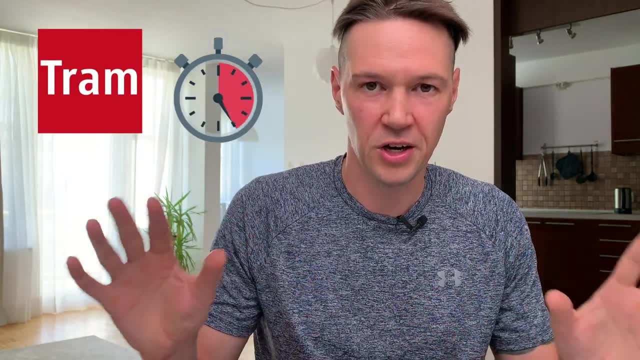 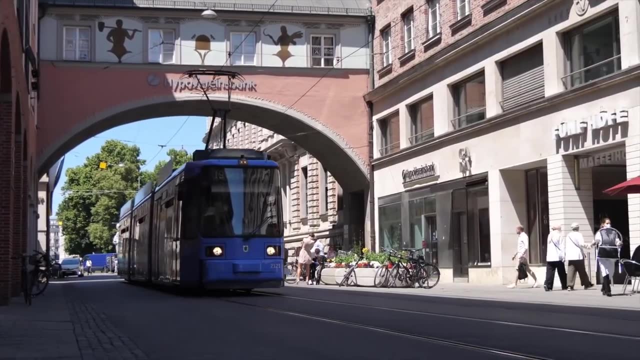 Trams, or in German, Nothing but Trams. This is Trams, Nice and relax way of cruising around Munich: Not very crowded, Big windows, And they go anywhere, Even to Bratislava. They go through really beautiful places of the city. 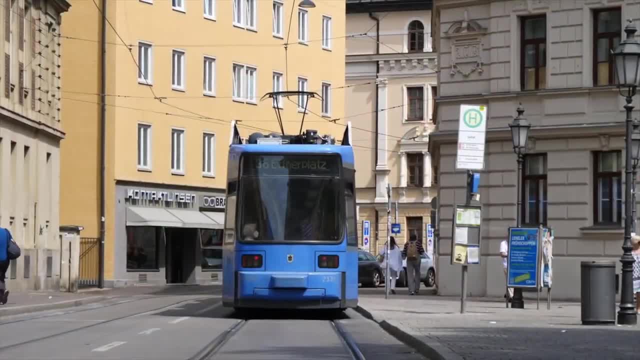 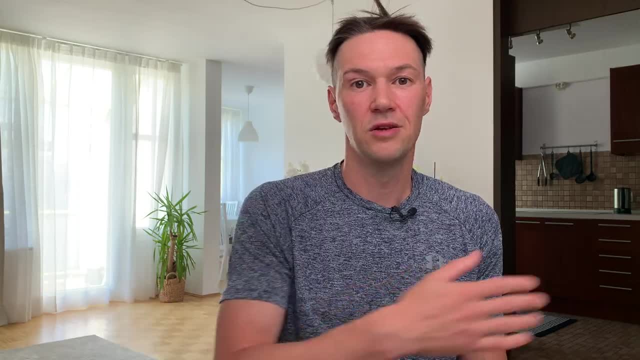 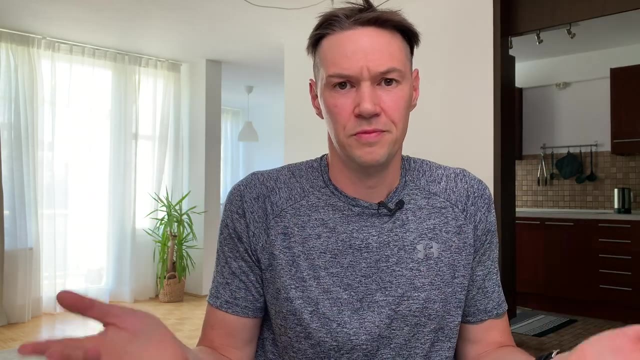 Just don't be surprised if the tram that you're taking suddenly ends on the middle of the route because of some building happening. Sorry, this is rails, They cannot go around. blocks, Magic And finally, buses. So this is buses. I don't know what to say about them. 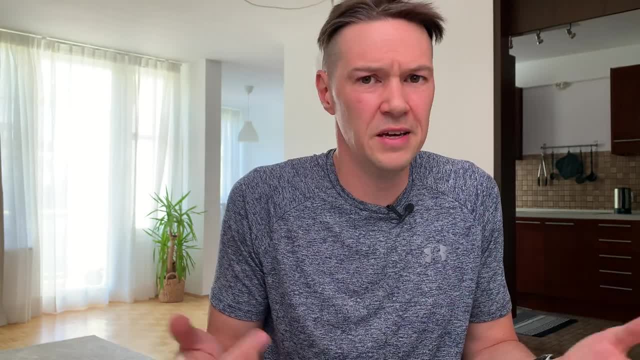 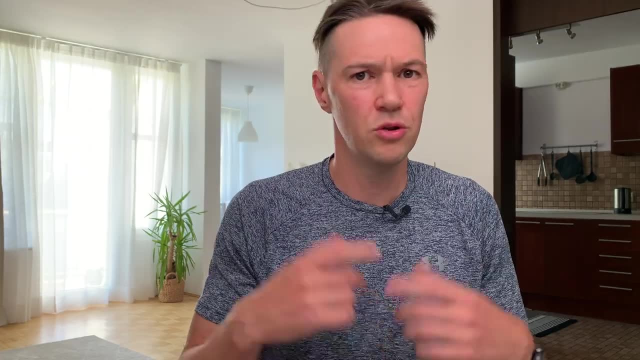 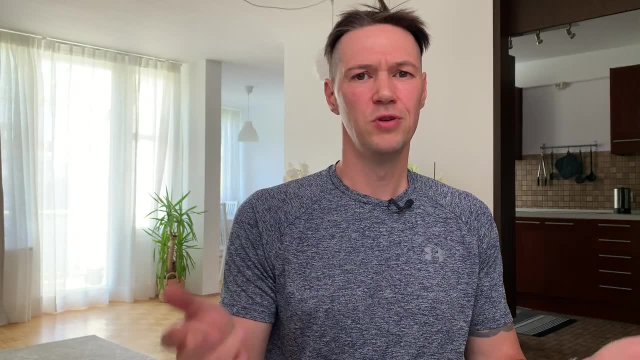 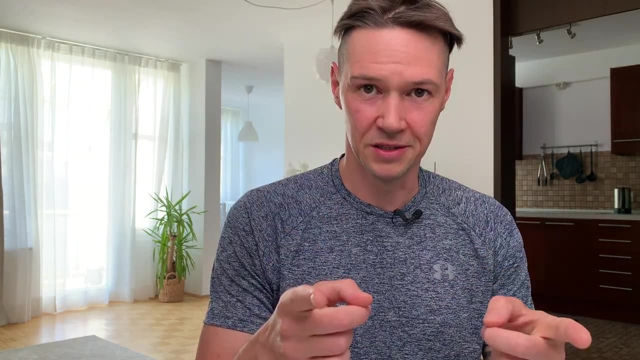 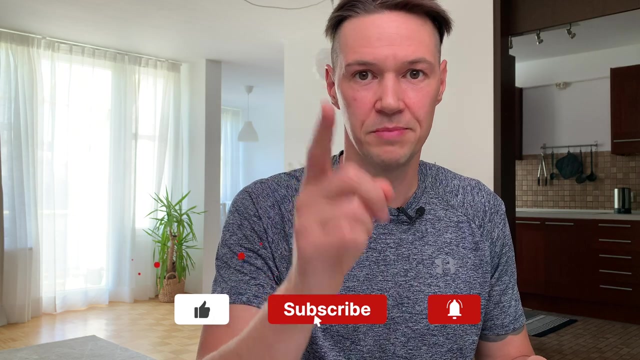 Now leave with this information. So this is all about navigating in Munich, public transportation and about public transport itself. Stick around and you will find another video about tickets. You will know what to do with all those tickets which exist in Munich. Thank you for watching. Like, share, subscribe. Bye-bye guys. You.